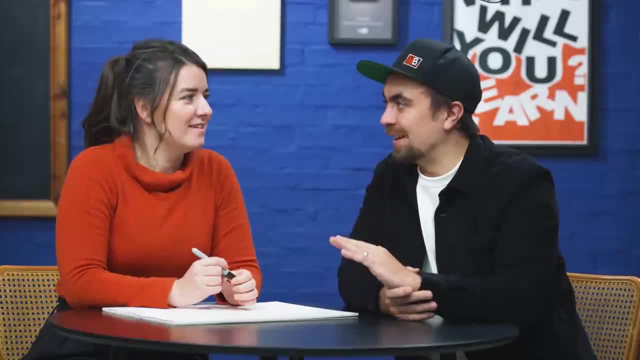 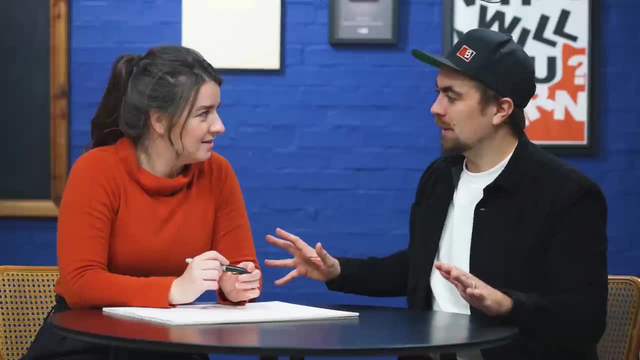 I've recently learned a new skill. I've not showed Kim yet and hopefully it'll blow her mind. Check this out. Okay, Kim, I want you to write down any random date that you choose. Write it in big letters on this piece of paper here. 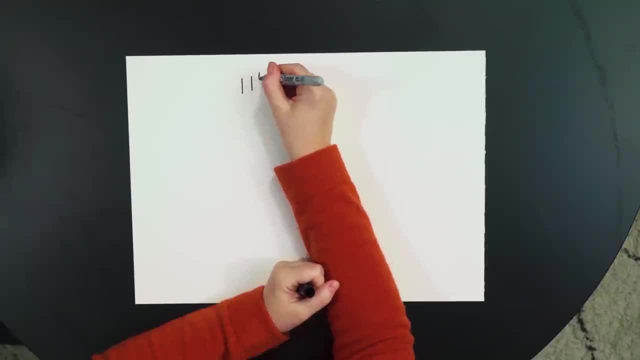 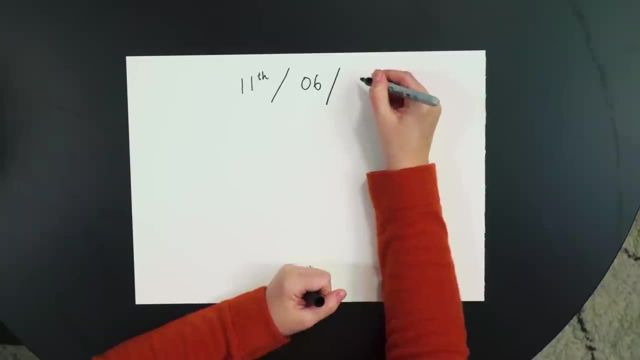 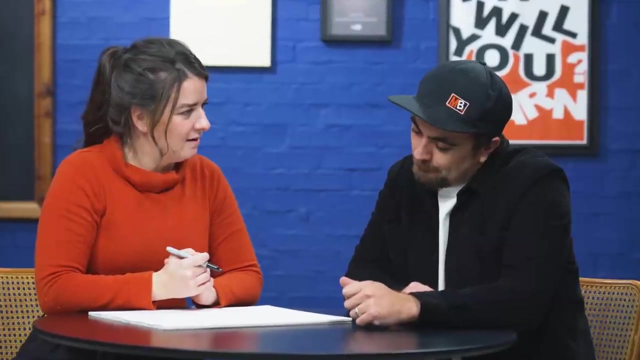 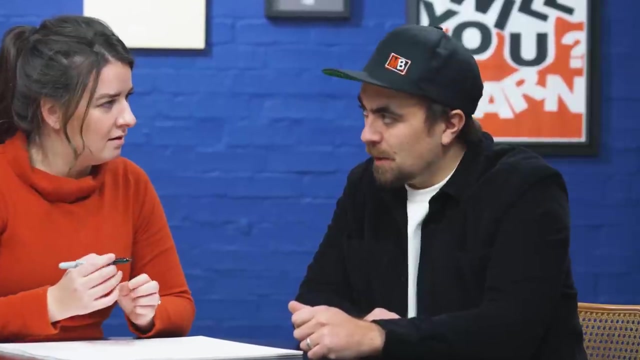 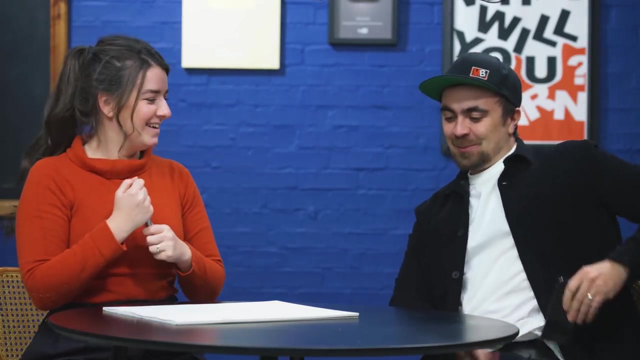 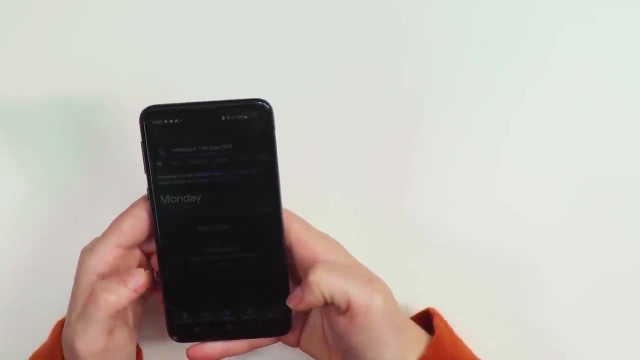 Okay, uh, the 11th of June 1973, That's a Monday, I don't know. Look up, Wait, where's my phone. 1973, It is a Monday. Pick another date. How did you know that? 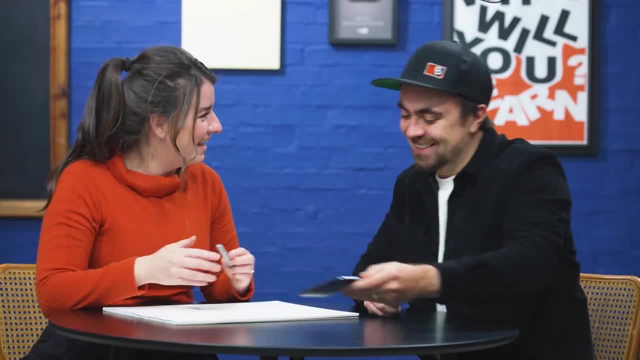 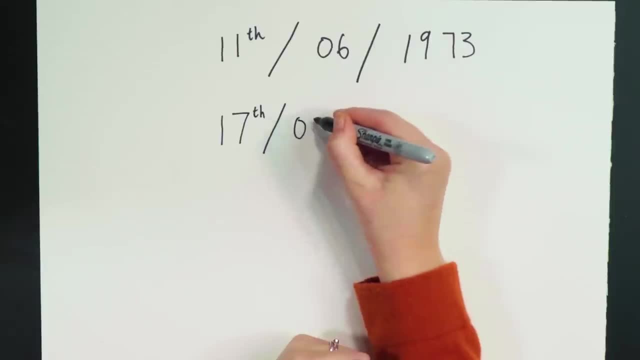 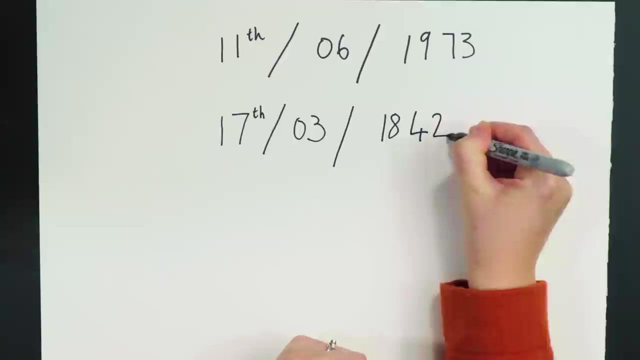 Pick another date. How did you know I would choose that date? I didn't know you would choose that date. Right, wait, put this away so we can. You're derring-browering me. 17th March 1842. 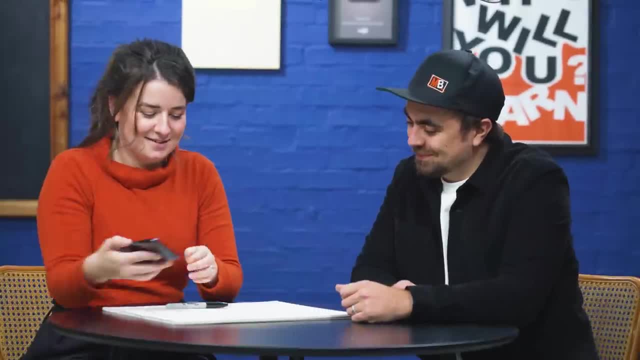 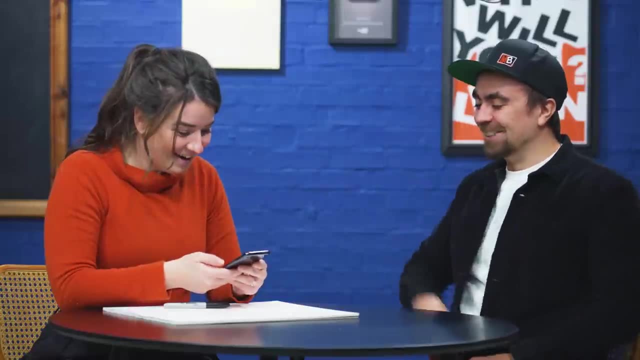 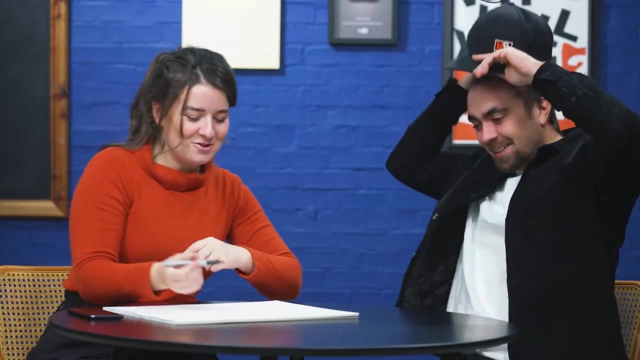 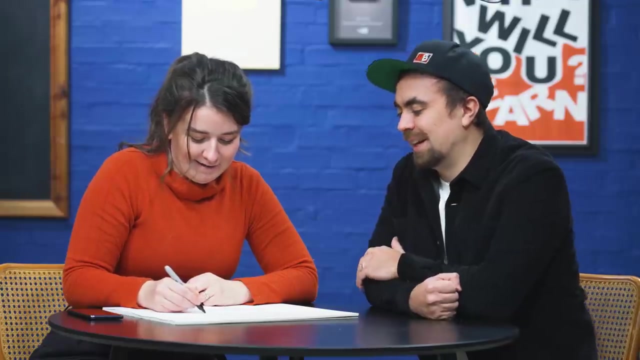 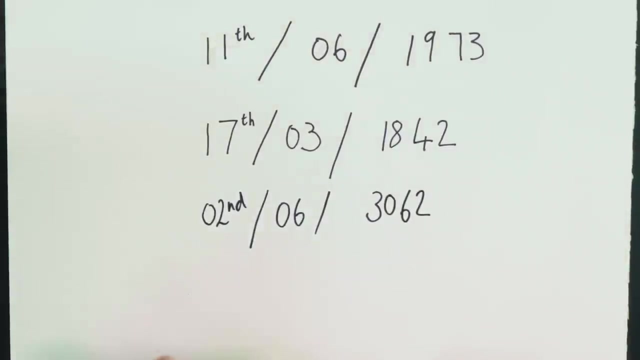 It's a Thursday, Thursday, Right, do one in the future. right, Do one that's not come yet. Any random date you choose, How are you doing this? 2nd of June 30, 62- Oh, that's a thousand years in the future, okay. 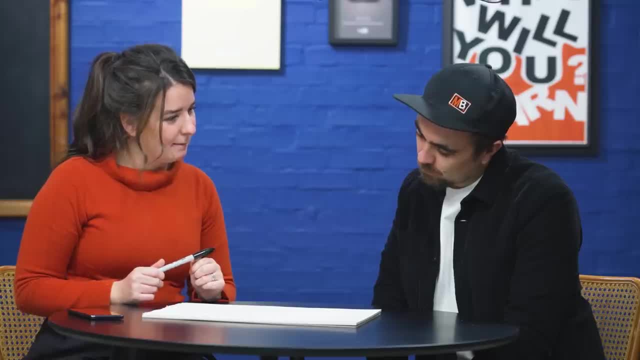 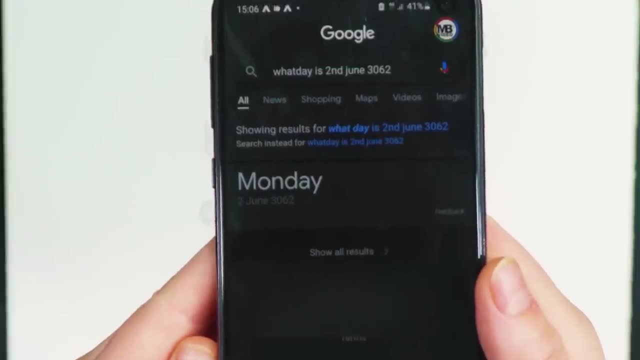 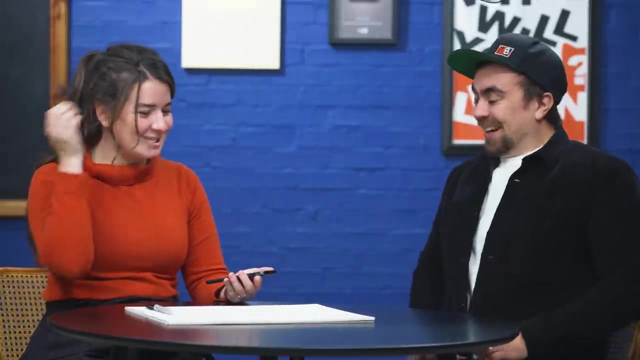 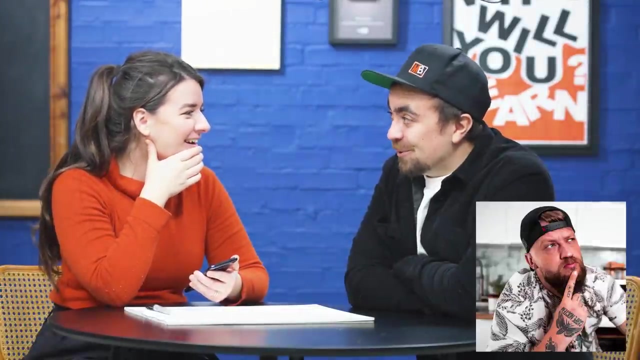 Right Monday, Monday, Oh my god, Pretty cool. eh, I'm so glad I got them right. Is this one of those? Is this like something that Chris Ramsey taught you? Uh, I bet Chris Ramsey knows how to do this. 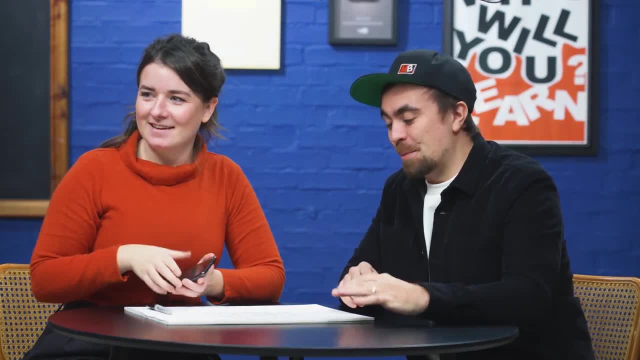 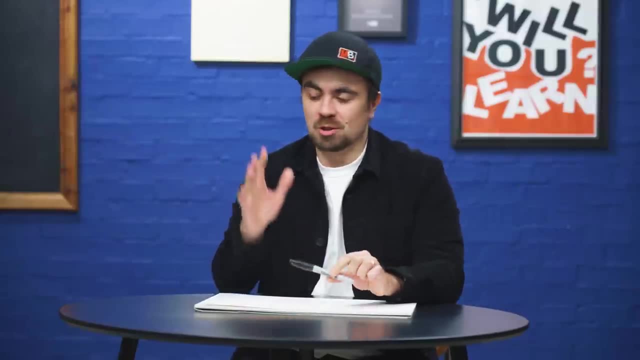 But it's not. It is not a magic trick, It's a legitimate math trick. That's awesome. I saw this skill or trick, whatever you want to call it- on Numberphile just a couple of weeks ago. James Grime, who is a mathematician who works at Cambridge. 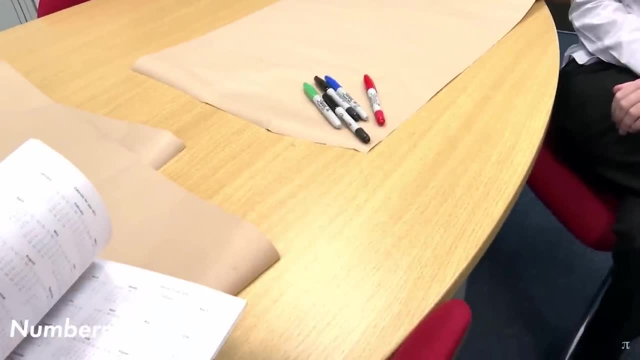 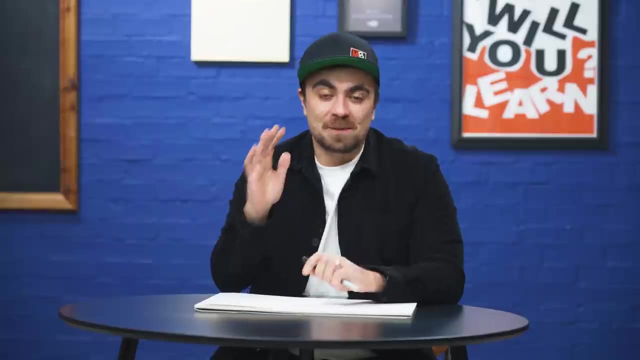 showed Brady Haran how to calculate the day of the week of any date- An arbitrary date basically- And he can do it really, really quickly just in his head. It's a fantastic video. It's linked below. The thing about James Grime is he's a mathematician from Cambridge. 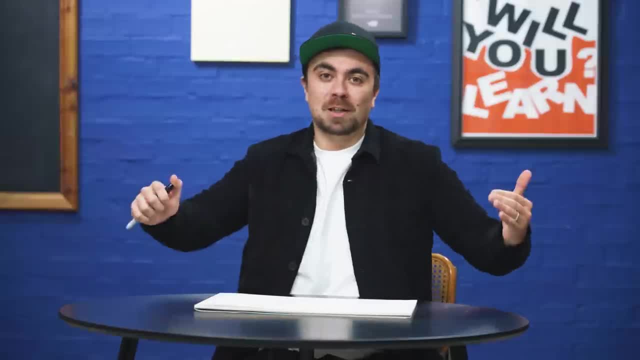 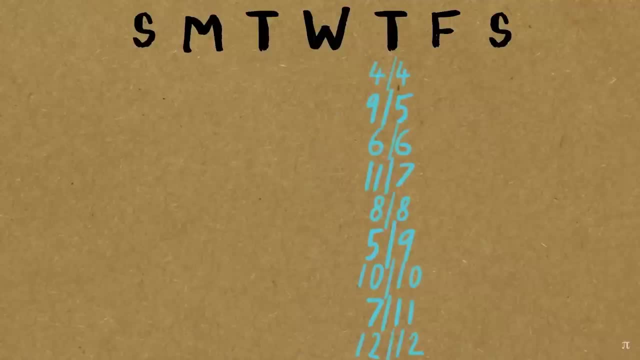 So he's a very intelligent dude, And that immediately made me think that I would never be able to do this. But I watched the video anyway and I kind of followed along with what he was doing, And at the end of the video I was still following along. 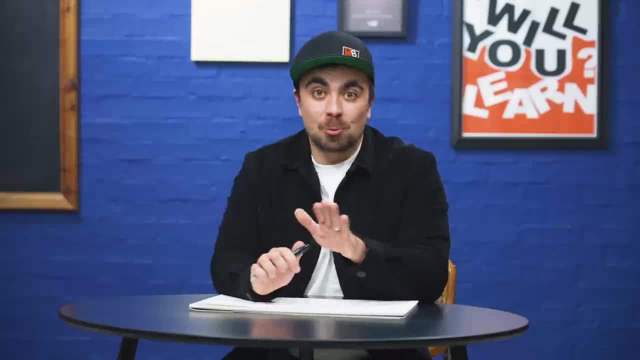 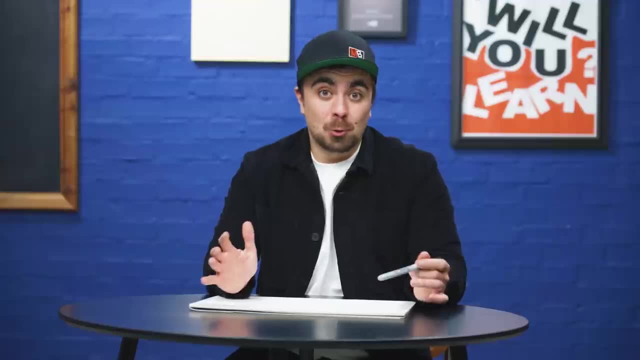 It didn't seem that complicated. I thought it would be amazing if I was able to tell people the day of the week for any date that they could possibly give me. So I thought I would give it a go, learning this myself, And it's actually not too hard. It all stems from a simple quirk in the calendar that we use. So basically, the 4th of the 4th, the 6th of the 6th, the 8th of the 8th, the 10th of the 10th and the 12th of the 12th. 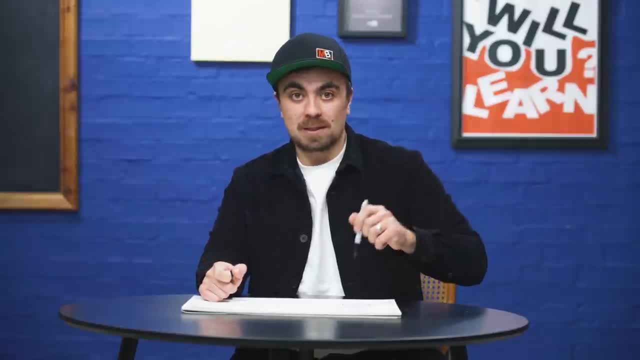 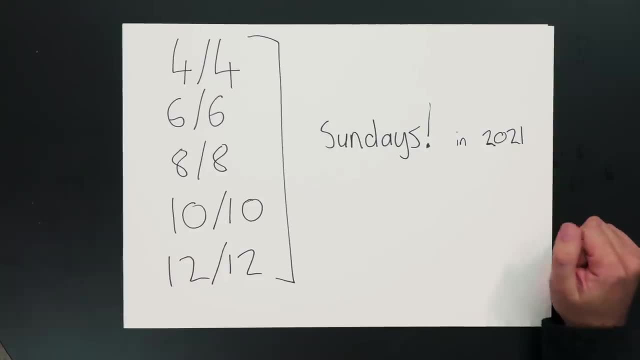 No matter what year it is, these all land on the same day. In 2021, these are all Sundays. So you can imagine if someone gave you the 6th of April, you would just add two days, So that's Monday, Tuesday, and you'd be able to tell people it's a Tuesday. 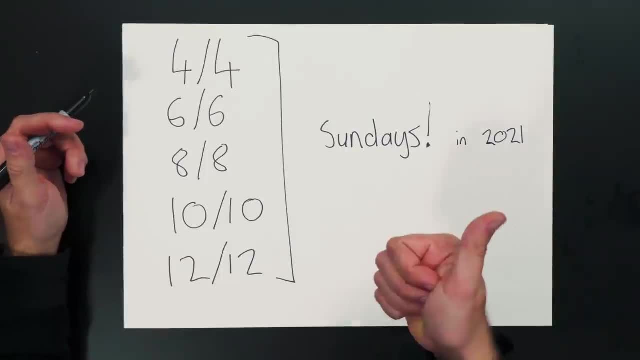 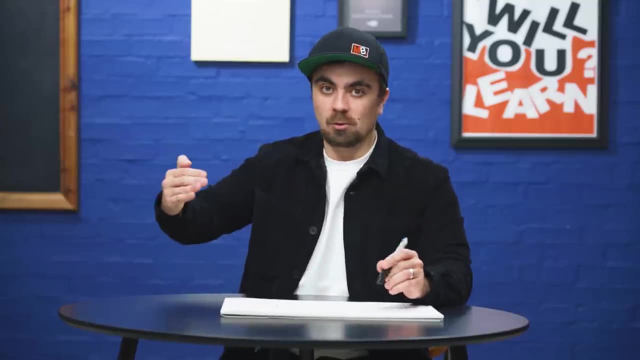 What about the 10th of June? Well, that's four days further on from here, So that's Monday, Tuesday, Wednesday, Thursday. If you can memorise these dates and you know that they are all a Sunday, then it's quite easy to work out what date you're given based on that information. 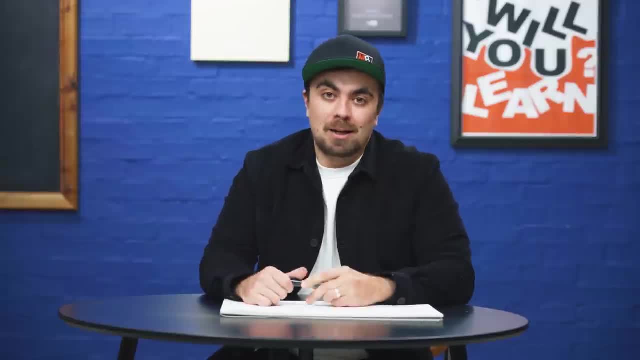 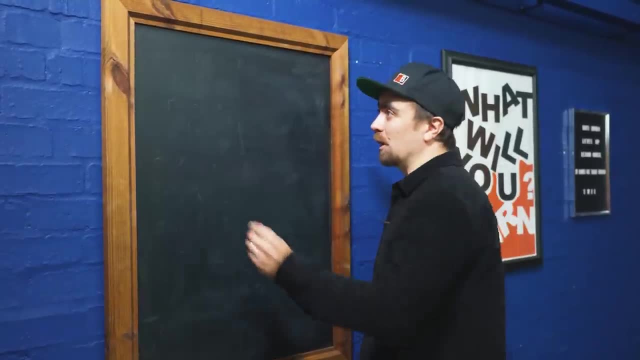 What about if the year is not 2021?? Well, this is when it gets a little bit more complicated. Let me explain. To make this whole thing a lot simpler, you first assign a number to each day of the week, So zero. 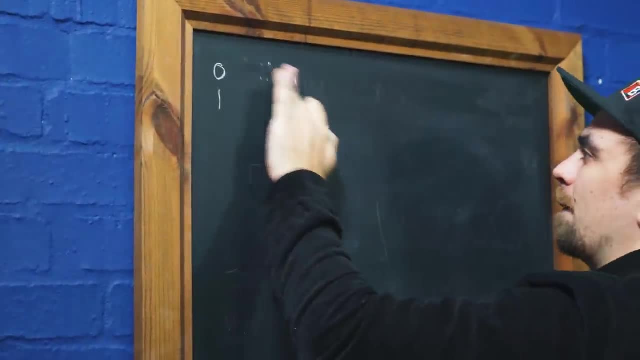 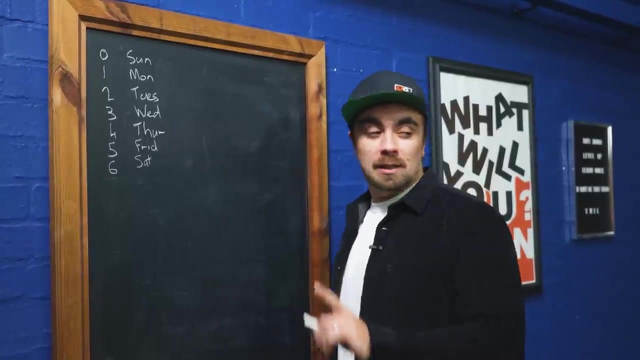 zero is Monday. No, zero is Sunday. Ignore that. One is Monday, Tuesday, Thursday. Then you need to work out what day of the week all those dates I spoke about earlier fall on for that particular year. That's a five. 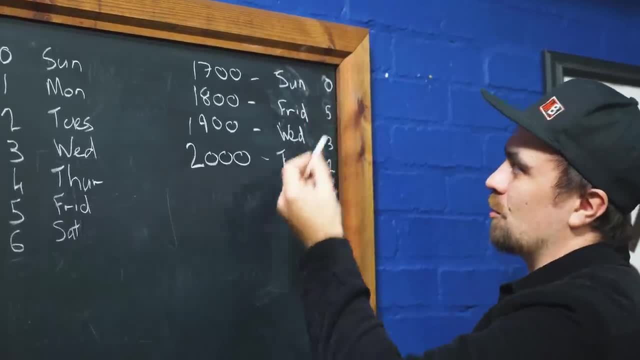 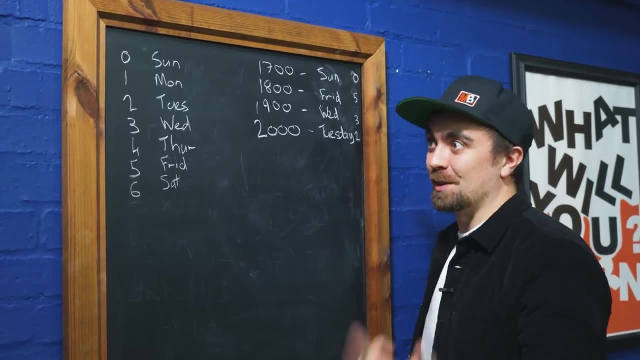 That's a zero. Oh shit, this is a Sunday. It goes Sunday, Friday, Wednesday, Tuesday. Sunday Friday, Wednesday, Tuesday. 2004 was a leap year, So you have to add five on The 4th of the 4th, the 6th of the 6th, the 8th of the 8th, the 10th of the 10th. 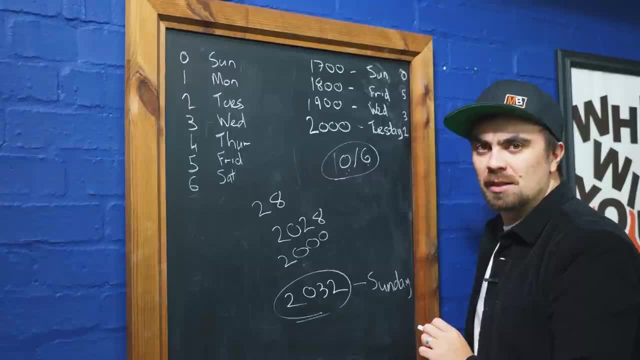 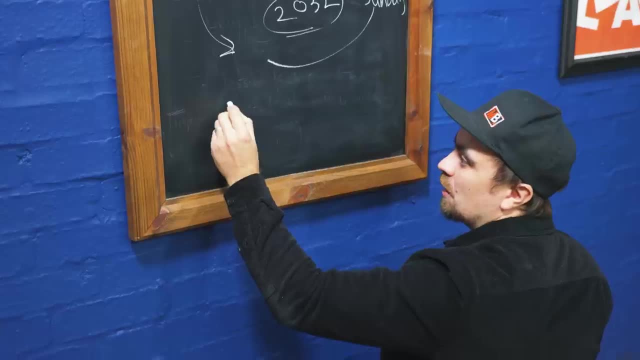 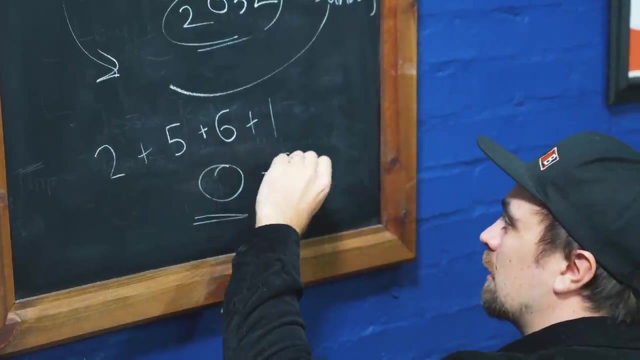 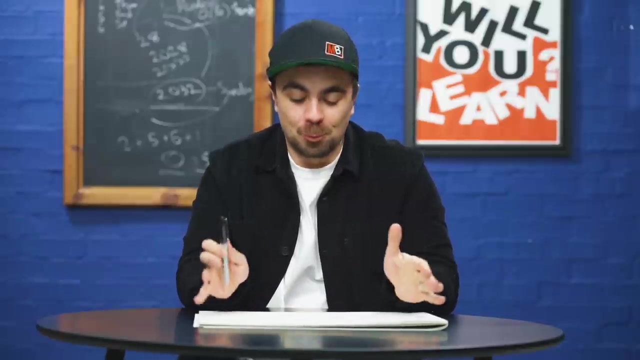 So in 28 years, what did I say Thursday? I said Thursday. So then you tunnel into the quantum realm. Two for a Tuesday plus the year, plus the number of leap years, is zero, which is equal to a Sunday. So clearly I'm really bad at explaining how to work this out. 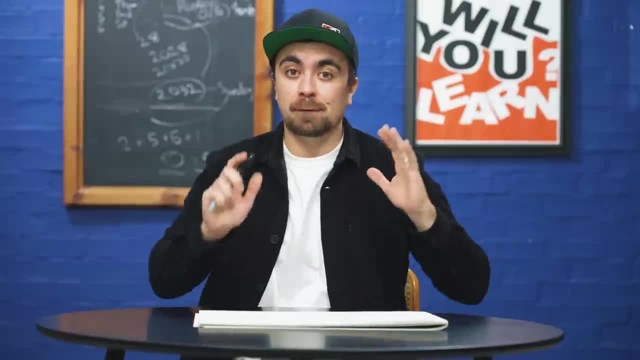 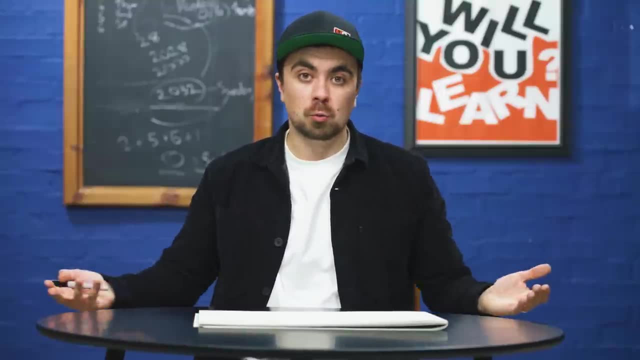 But trust me, it's not that difficult And James Grime did a fantastic job of explaining it in layman's terms. On the original Numberphile video, I was able to follow along one or two watches and I was calculating the days of the week. 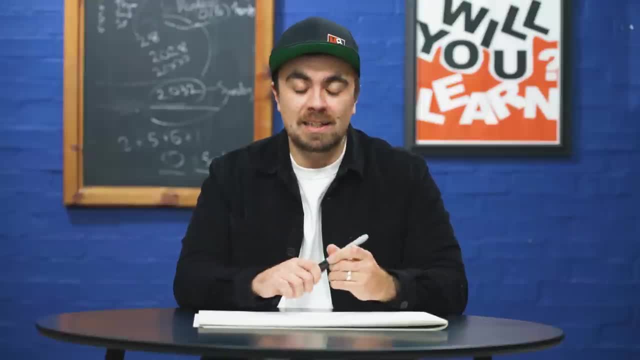 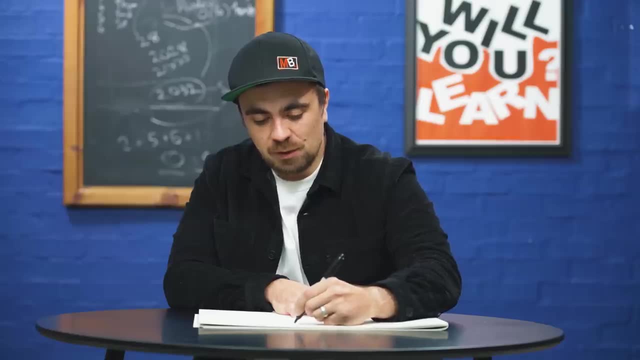 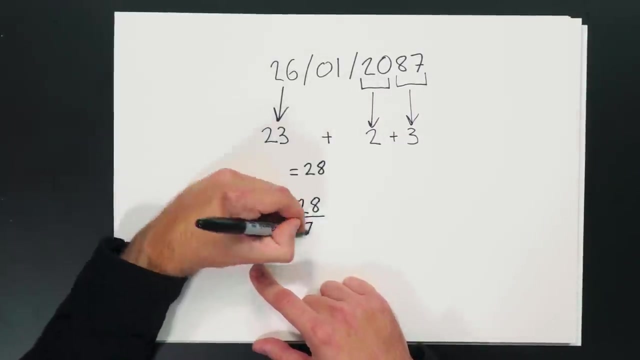 of any arbitrary date. Basically, the technique he uses reduces a date like the 26th of January 2087 down to just a simple sum With a pen and paper. this sum is really easy to work out. The difficult bit is trying to do it in your head whilst having a conversation and not 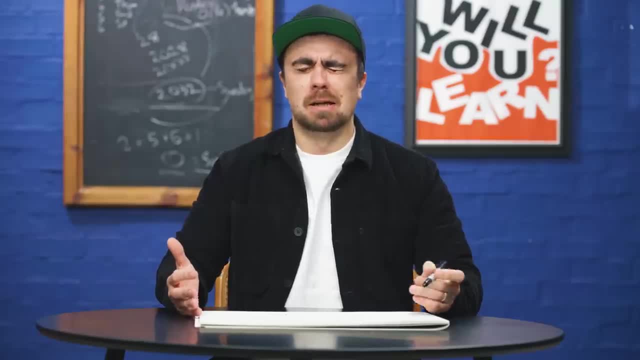 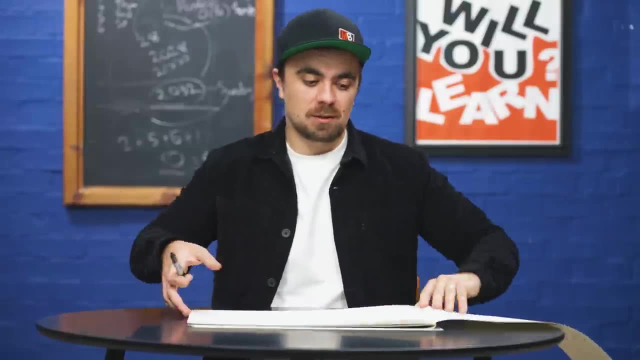 just being like 24 plus three, So easy to do, difficult to do at speed. So how did I learn? Well, first of all I wrote myself out my cheat sheets, which give me all the days that fall on the same day of the week in the calendar. 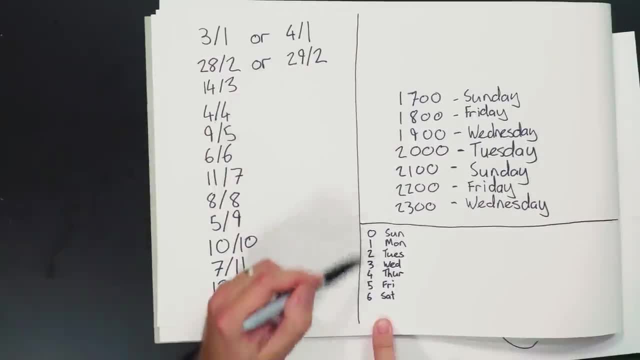 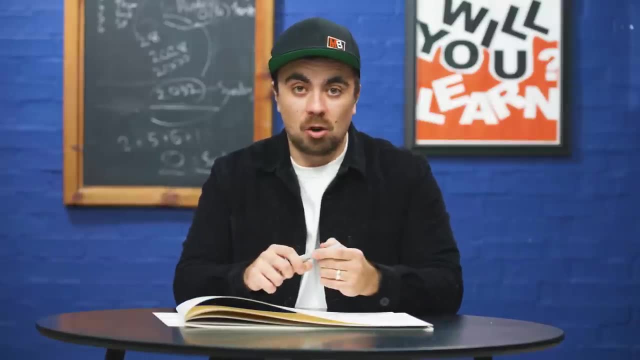 Then I wrote out the century starting points for me And also in the corner, the number corresponding to the day of the week. So I set this aside and just started practising on dates with a pen and paper, trying to work it out. 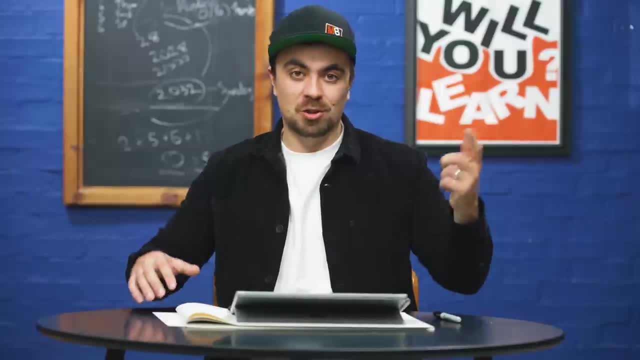 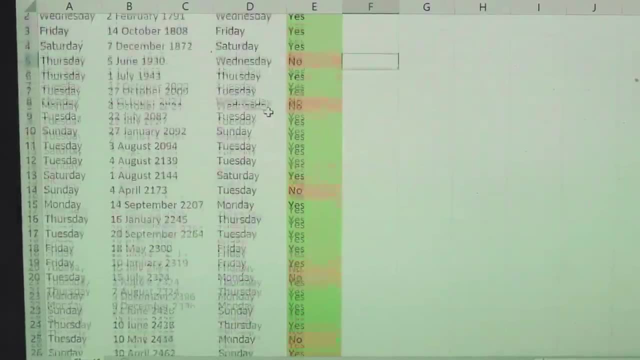 I actually have a spreadsheet. I actually use the spreadsheet. It just generates random dates And then I put in what my guess was and it told me whether I got it right or wrong. So you can see, at the start I'm pretty frequently wrong. 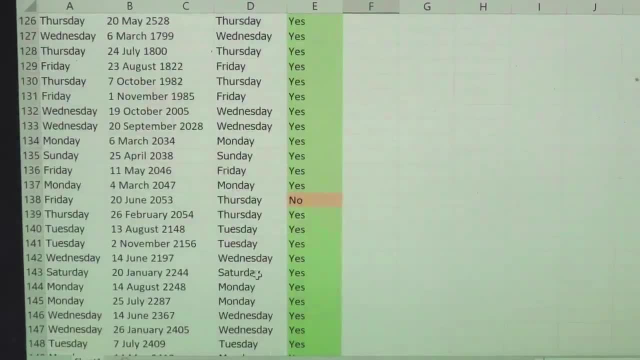 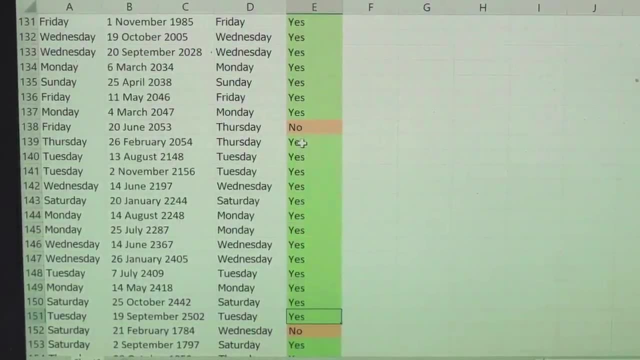 But by the time I'd done this 142 times, I had a string of 1,, 2,, 3,, 4,, 5,, 6,, 7,, 8,, 9,, 10,, 11,, 12,, 13, 14 straight correct guesses. 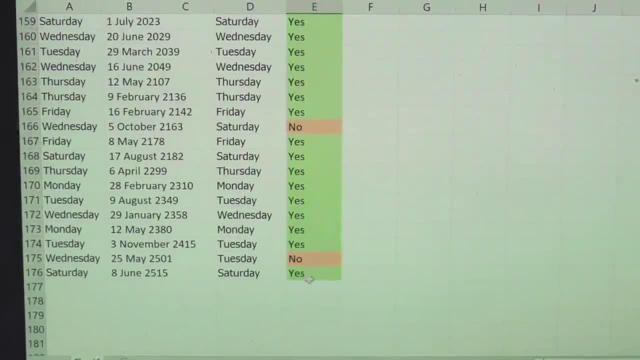 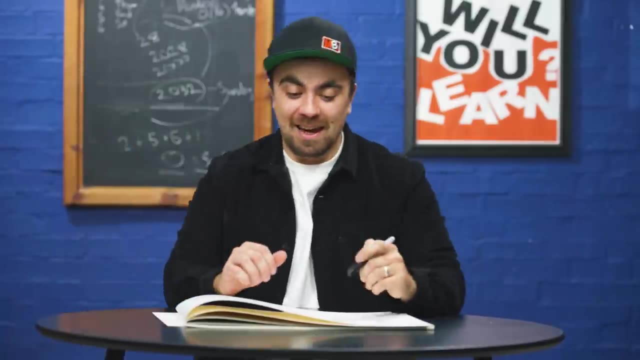 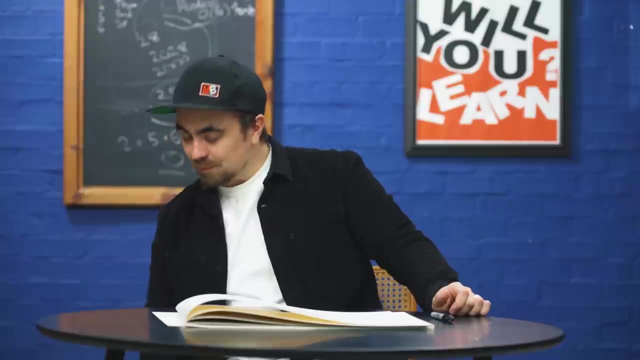 So I was getting pretty good at it And I did this a total of 176 times. So I sat with headphones on on a Friday night and a Saturday morning and just guessed 176 dates. Wild weekend, Yeah. Halfway through I ditched the pen and just started doing it in my head.